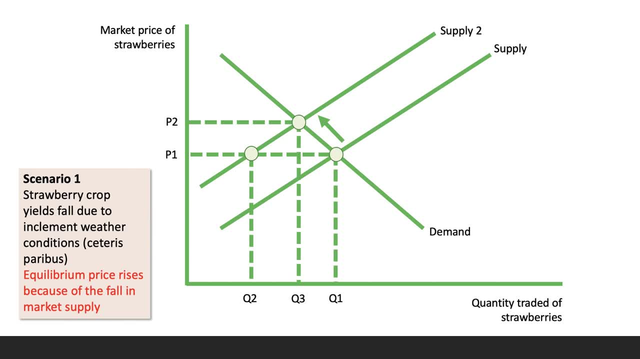 Price will rise eventually from P1 to P2 and the market may settle at a quantity traded Q3. So this makes intuitive sense, is it not, that if there's a poor harvest, you'd expect to see the retail price of strawberries go up. Higher prices help, in this instance, to ration demand. 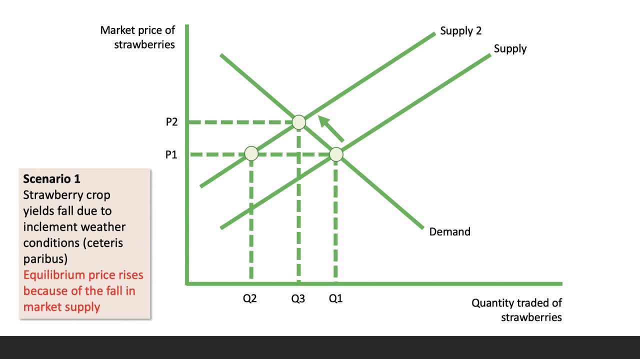 when perhaps there's a shortage of available supply. Here's our second scenario. The government campaigned successfully to promote strawberries as a low-priced product, but the price of strawberries went up and the price of strawberries went down. This is a low-fat, healthy food. Same initial situation: price: P1, Q1.. In this situation, 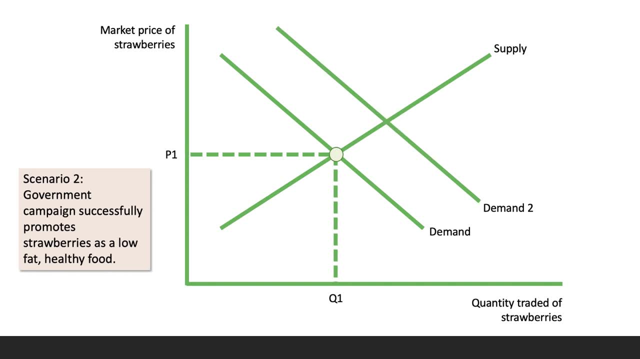 we'd expect demand to shift out. Successful marketing campaign will increase the total number of consumers willing and able to buy strawberries Again. if the price stayed at P1, this time, there will be excess demand in the market And again there's pressure, this time for the price to go up. The new equilibrium is at P2, output Q3, where demand D2, demand curve 2, intersects with supply. The increase in demand causes an expansion of supply and a rise in the equilibrium price Over time. higher prices for strawberries, for example. 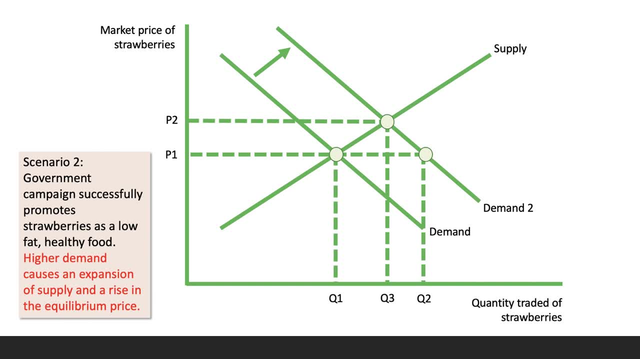 that would act as a signal to growers to attempt to expand their production in future time periods. So high prices, or higher prices in this situation in price rising from P1 to P2, can stimulate supply through what economists call the profit motive. One more scenario for you in this video, Here's: 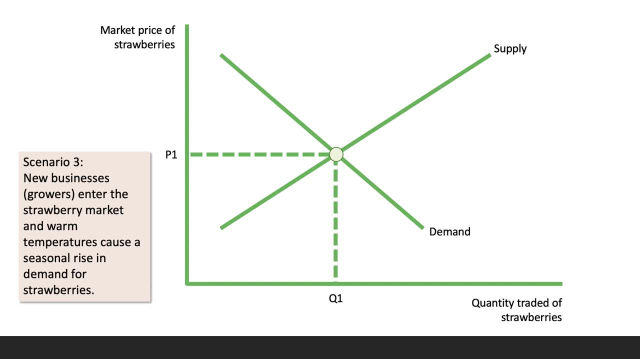 scenario three: New businesses or new growers enter the strawberry market and warm temperatures cause a seasonal rise in demand for strawberries. So it looks as if we have two factors here, One affecting supply and one affecting demand. Which way do you think the curves are going to go? 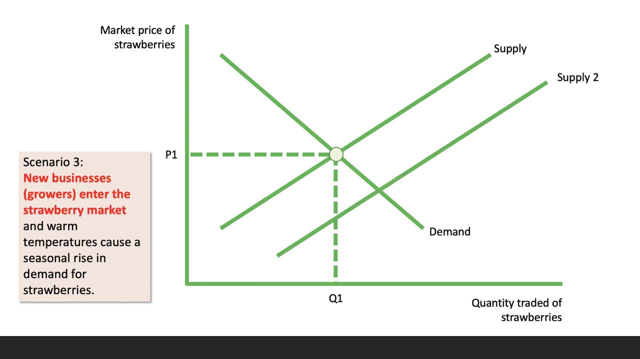 Well, let's take them in turn. If new businesses enter the market, then the market supply curve would increase. There'd be more strawberries grown and supplied to the market at each price. Warm temperatures will cause an increase in demand. Seasonal demand for strawberries will. 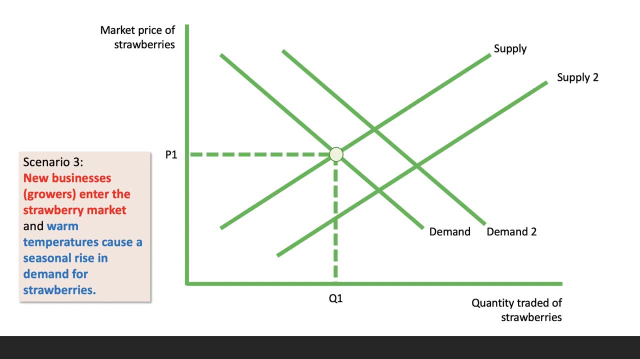 be higher as people enjoy their strawberries and cream in the summer months, So the demand curve might shift to P1 and P2.. So there's an increase in demand for strawberries. There's an increase in demand for strawberries and cream in the summer months, So there's a shift out from P1 to P2 demand.